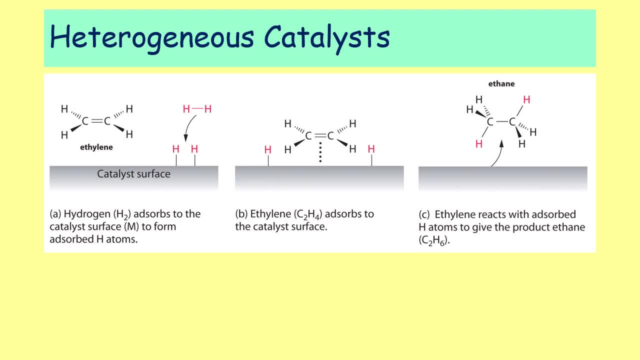 to the reactants. Usually in these situations the catalyst is a solid and the reactants will create bonds to the surface of the catalyst. So the reactants in heterogeneous catalysis reactions adsorb. So I have not spelt that word incorrectly, It is. 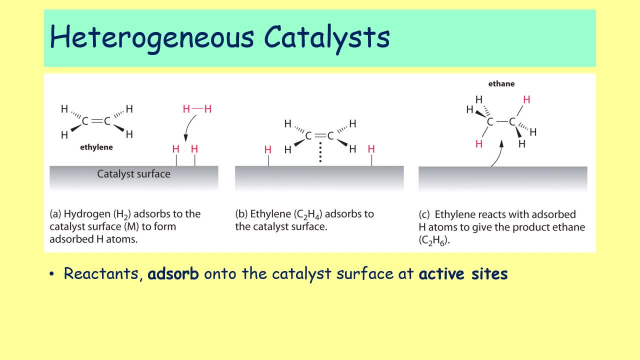 supposed to be spelt with a d That adsorb means that they're only on the surface. They're not going the whole way into the catalyst, because the catalyst is solid. They are only adsorbing onto the surface And the points at which they adsorb on the catalyst are known as active sites. Very, very. 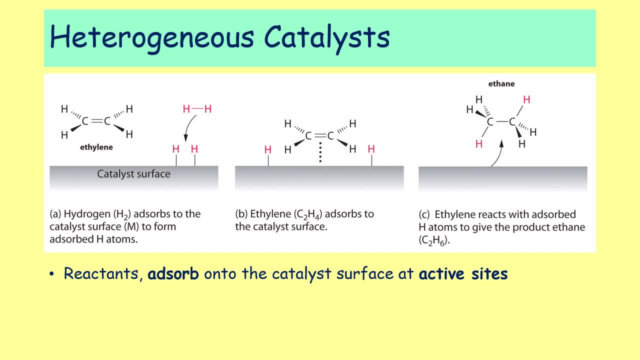 similar to how an enzyme has an active site: a part of the enzyme that the reaction takes place on The part of a transition metal surface where the reaction takes place is the active site. Now what happens is that you do get an active site. 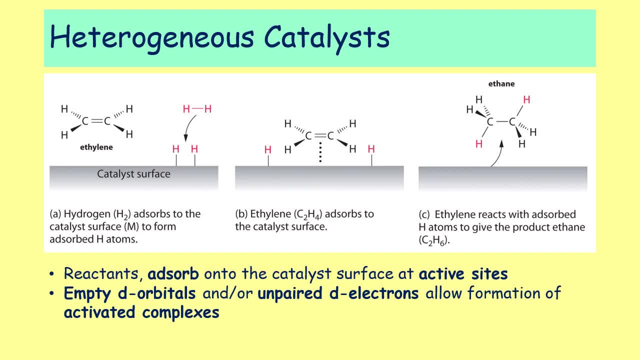 You do get slight bonding and this is between empty d orbitals on the transition metal or unpaired d electrons, and this creates an activated complex. Remember, every reaction has an activated complex and the activation energy is the energy needed to achieve this activated complex. Catalysts provide an alternative path. 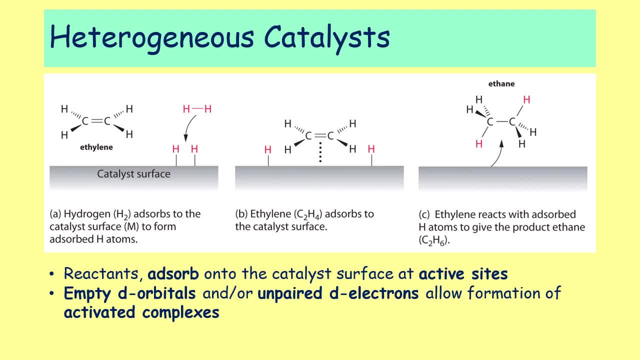 And they provide an alternative pathway by allowing a different activated complex to form. And this different activated complex involves a level of bonding between the reactants and the d orbitals and potentially d electrons, the unpaired d electrons- on the catalyst surface. It lowers the energy pathway compared to the uncatalyzed reactions. Now, what you've got to? 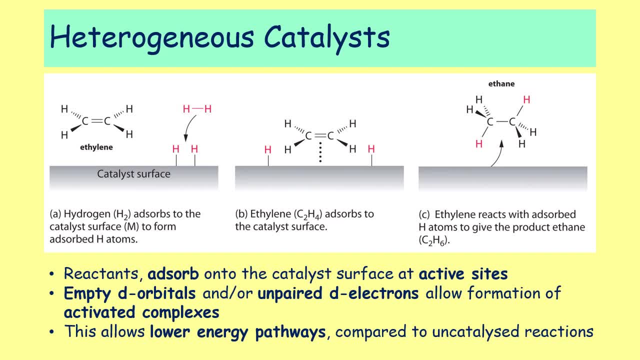 remember with a heterogeneous catalyst is that once the reaction has occurred, the product molecules need to then leave the catalyst surface, so the catalyst surface can be reused over and over and over again. If molecules bond to the surface of the catalyst and do not go away, that catalyst will not be useful anymore because active sites will be blocked. 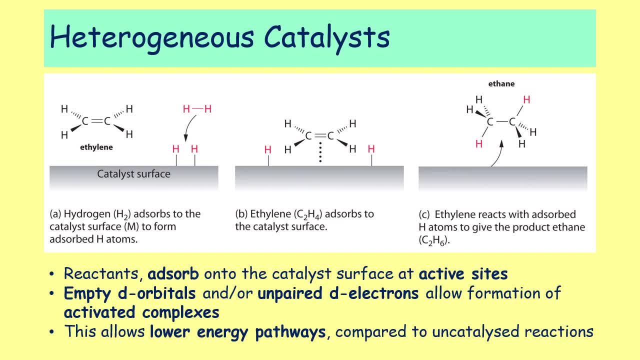 We would describe that catalyst as now being poisoned. So it is important with heterogeneous catalysts that you know the reactants are adsorbing onto the surface at places known as active sites. You are creating activated complexes through bonds or interactions between the d orbitals of the catalyst. 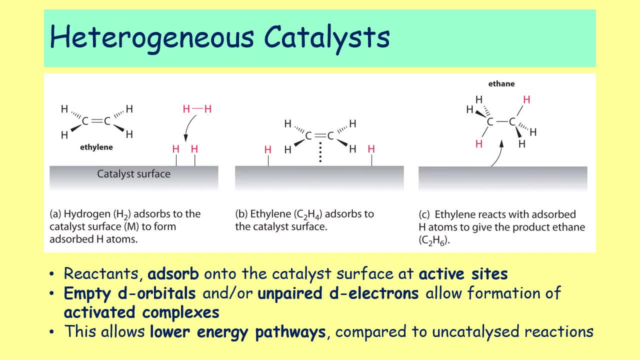 and the orbitals- molecular orbitals- of the reactions, You're creating a lower energy pathway. and when your reactant is sorry, when your reactant has been fully converted into your product, that product leaves the catalyst active site, so the active site can be reused. 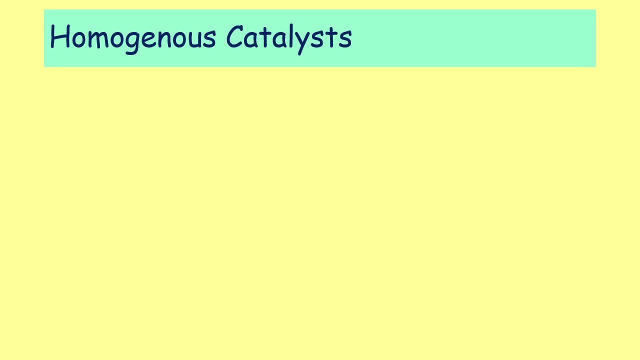 The second type is homogeneous catalysts, and typically at advanced, higher homogeneous catalyst, We are going to be thinking about a catalyst that is insoluble, And we are also going to be thinking about an insoluble catalyst that is seems to be expected to be react in active form. 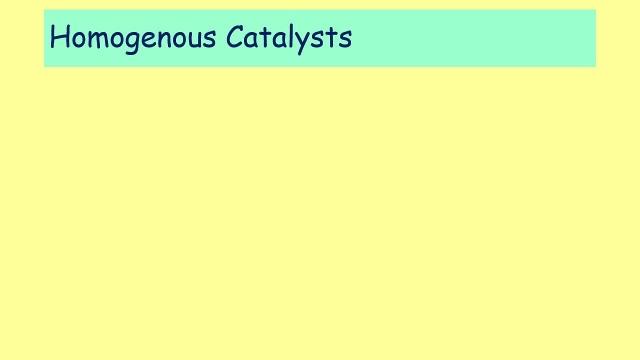 in solution and the reactants are also in solution And typically our homogeneous catalysts are going to be transition metal complexes. Now what happens in this case is your reactant molecules replace or substitute some of the original ligands that were on a transition metal complex. So you're replacing some of your ligands with reactant molecules. 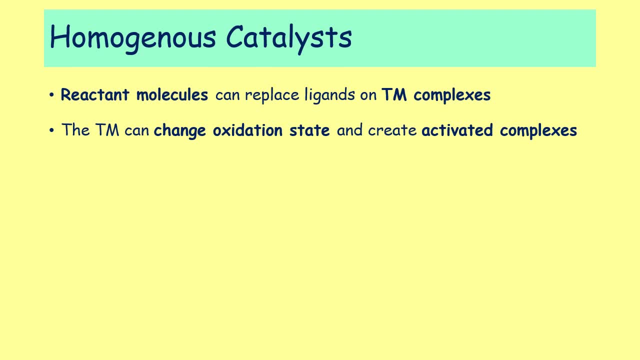 The transition metal can change oxidation state and create activated complexes. So make sure you're using this word activated complex, because that's what every reaction goes through, And what's happening is often an oxidation or a reduction between the ligand, the new reactant.